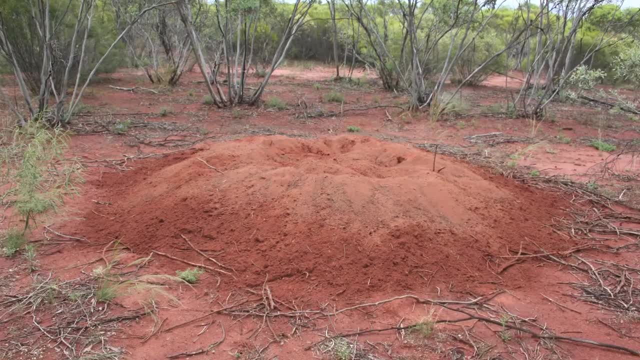 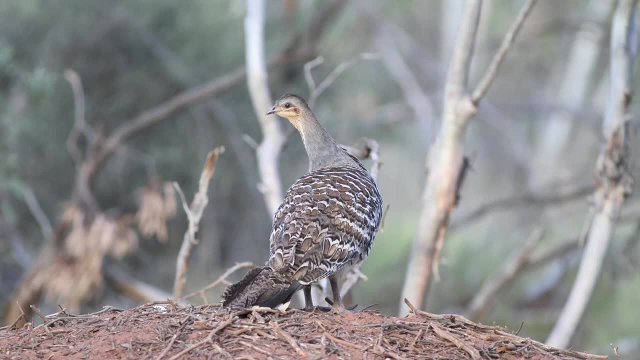 up and put them in the trailer and bring them back to here. It's more so with the birds effect, with the malleefowl and that, so they're damaging the nests and so we like to get rid of them and that way we can still have the malleefowl around. and yeah, they just disappeared. 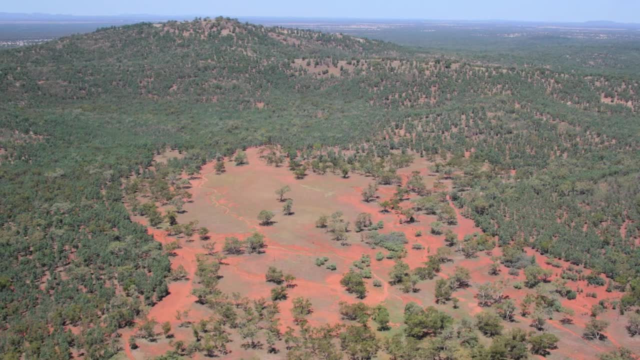 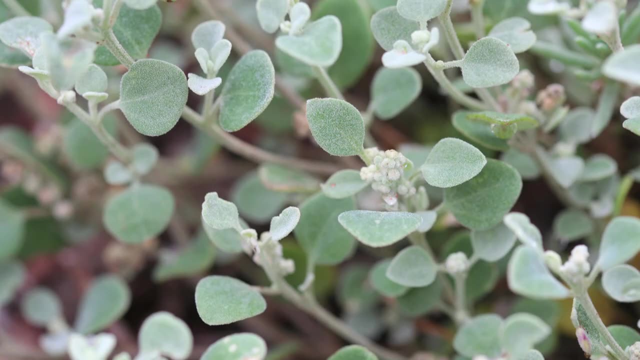 you know like there's a lot of land clearing and that's what knocks them about quite well, and all the goats seem to. you know, just browse and everything what the malleefowl are browsing on. so we're trying to get rid of the goats and keep the malleefowl, The goats they tend. 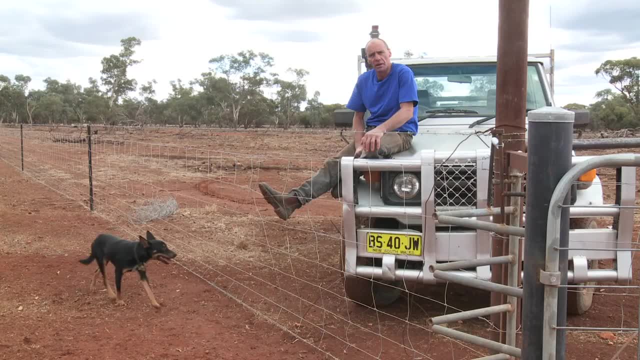 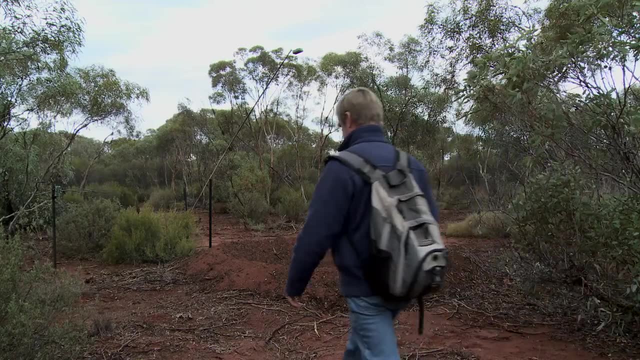 to jump on the mounds and they knock all eggs and that around and the malleefowl don't want to go back near them and that's why we want to get them out of there so they're not jumping on and knocking the nest around. 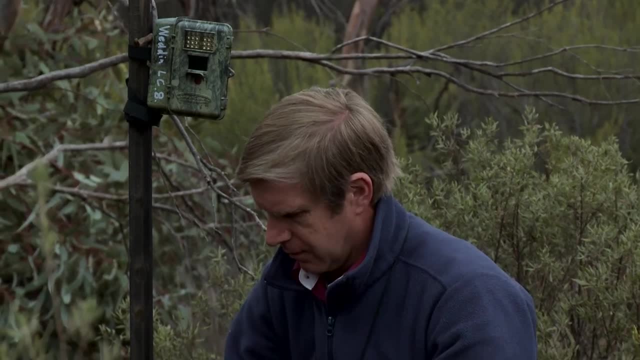 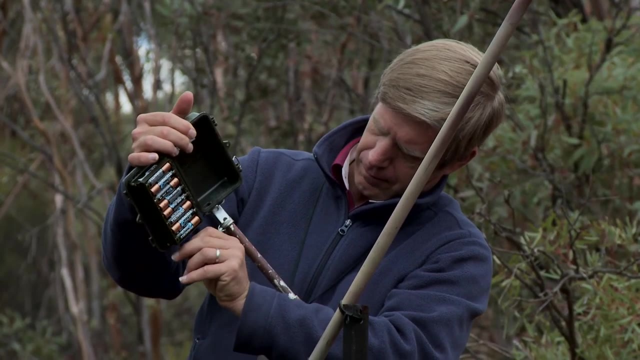 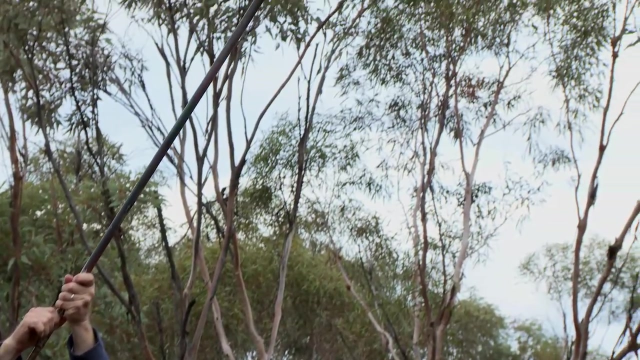 Starting in early 2000 I began a career of really conservation based projects where I looked at threatened species right across Australia and worked with landholders and the community to put in management strategies that would help all of those threatened species. A lot of malleefowl still exist on private land. 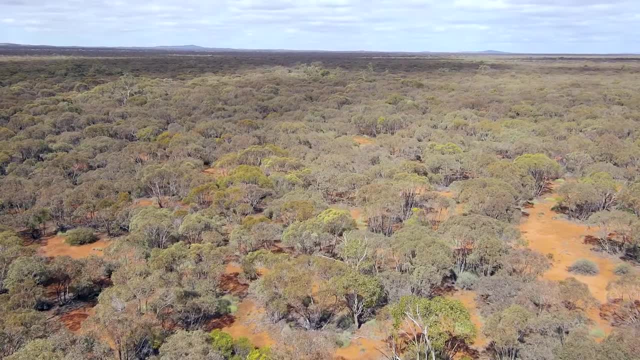 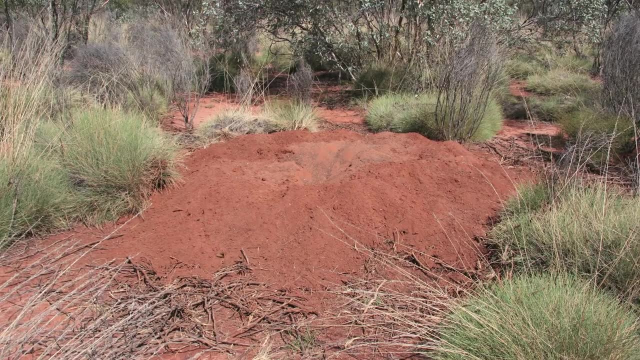 And because they're on private land, it means that actually the private landholders are doing something right. These birds wouldn't be here if it weren't for good management by these people, So I've wanted to look at how they're managing their land. why the birds? 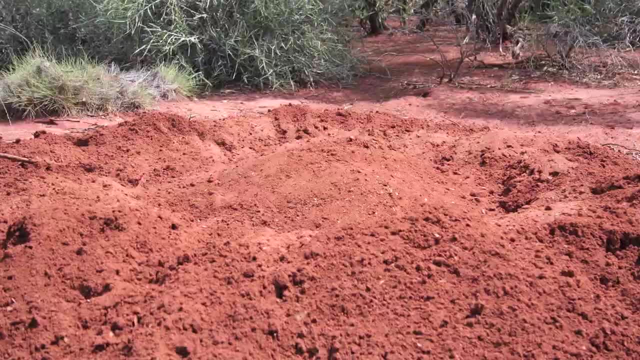 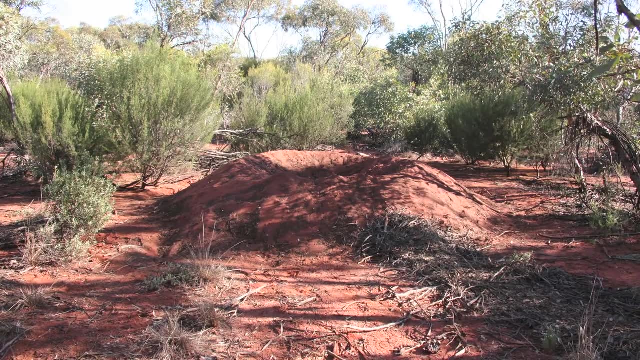 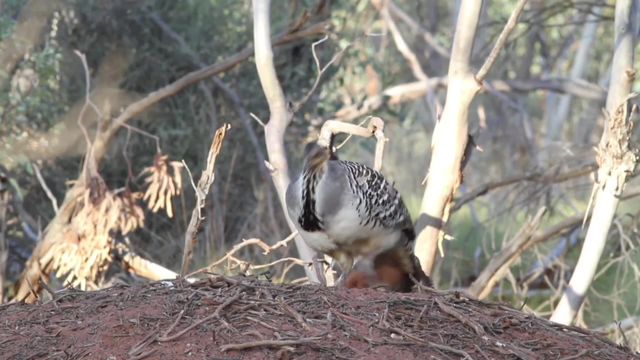 are still here and if there are any aspects creeping up on these birds that we might not be aware of yet, that could lead to future problems. Malleefowl are fantastic birds. They are incredible. The male in August comes in, he digs a huge hole which he then proceeds to fill with debris. 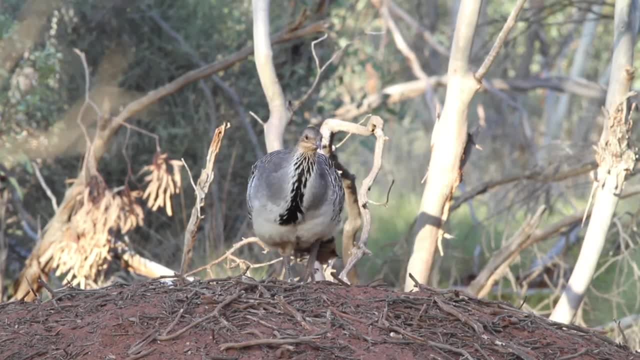 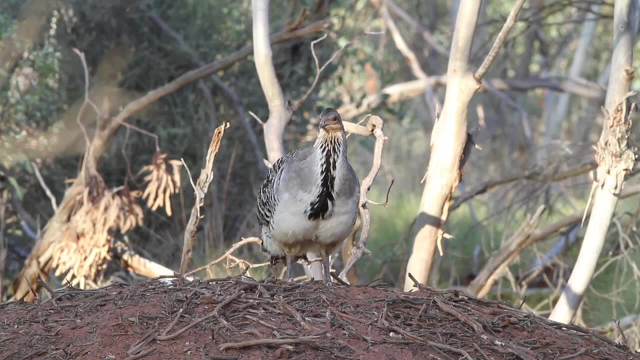 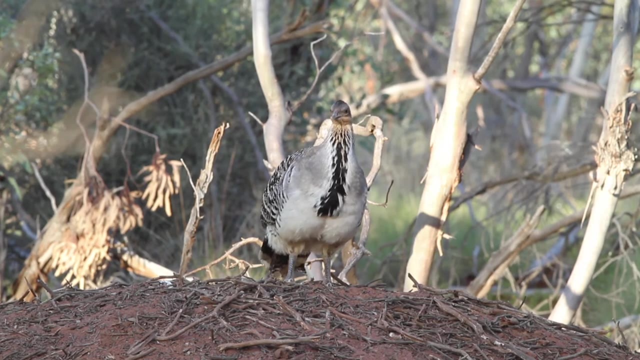 from around the nest, so leaves twigs, sticks and creates a compost heap. And then, when it's ripe, the hen comes in and starts to lay her clutch of eggs. Depending on the season for these birds, they vary how many eggs they lay. So in bad years, when perhaps there isn't, enough rainfall. They have smaller clutches of eggs- maybe six- But in the really good years they step up production and they might produce 20, even 30 eggs in a single season. So where we see the wheat belt through New South Wales now was where mallee were most. 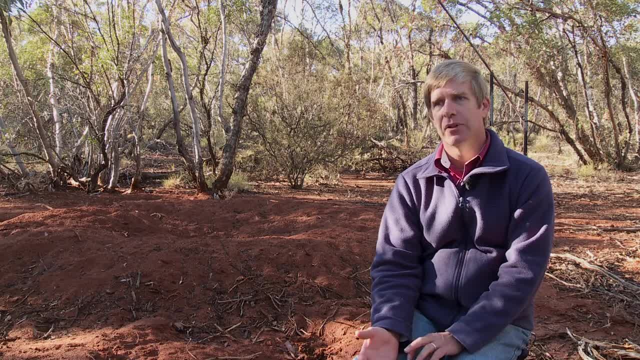 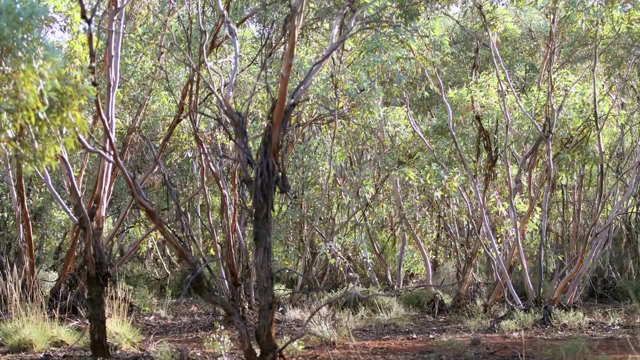 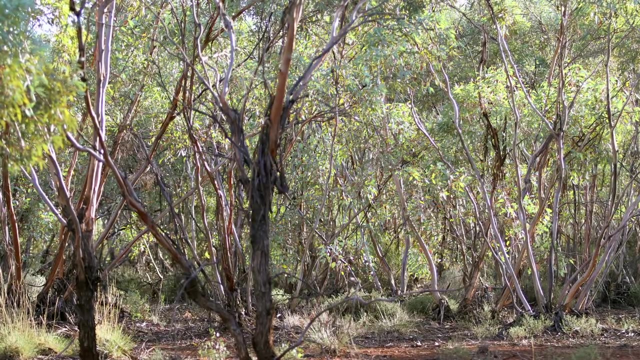 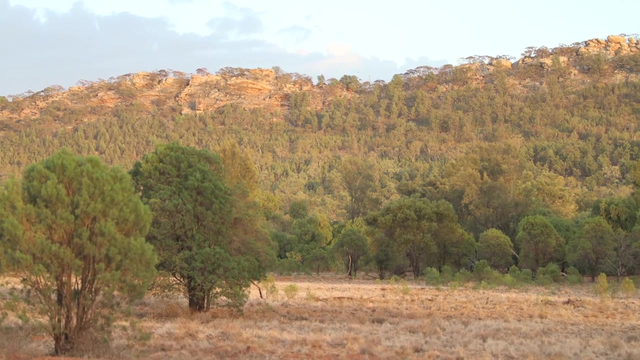 productive, The most birds were seen in those sites. Now they're restricted to less productive areas such as mallee woodland, So we don't see as many birds now either, Because they're not in places that were typically suited to them. My largest malleefowl part of the project is located around Mount Hope, where I have 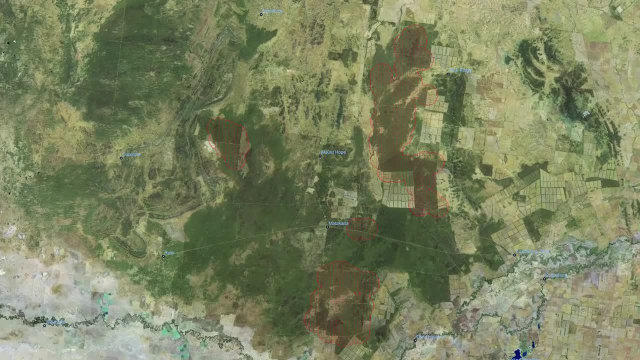 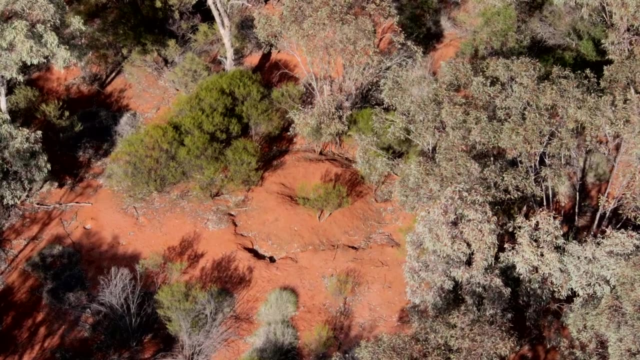 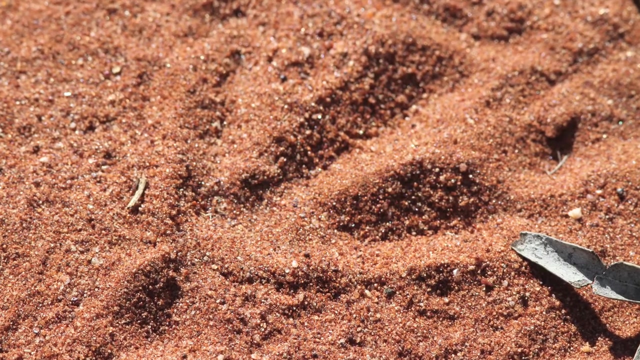 about five landholders that have populations of birds on their land. I also have a small population near Rankin Springs. It's very small and still dwindling. I have another population at Yalgogarin. It's one of the largest populations in New South Wales, But that's now been reduced. 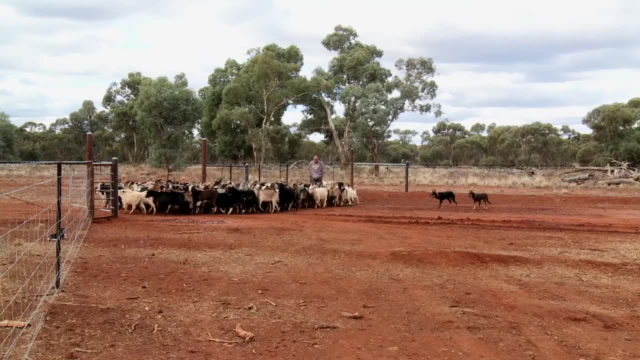 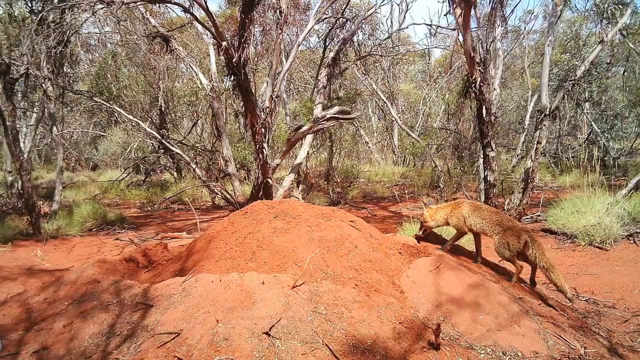 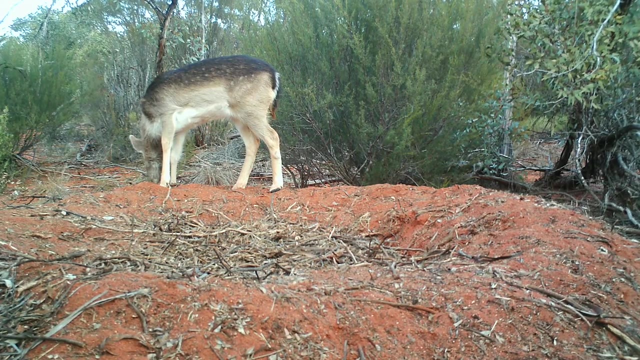 to only two, perhaps three breeding pairs. Each of the sites has a different problem, So the Mount Hope area has a lot of grazing with goats, Whereas Yalgogarin has foxes, And in the Rankin Springs area they have a problem with pigs coming in and digging ground. and removing vegetation. 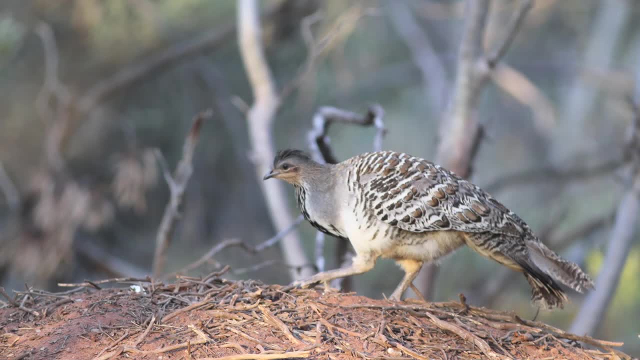 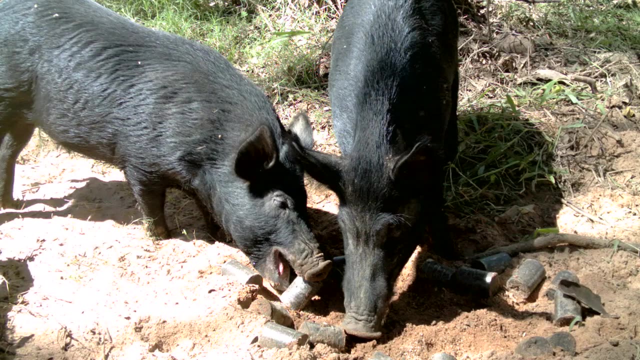 I grew up on a farm also interested in, I guess, native wildlife and their conservation, and pest animals are one of Australia's biggest threats to the conservation of native species. So feral pigs impact the environment through a number of ways, but the key ones would be: 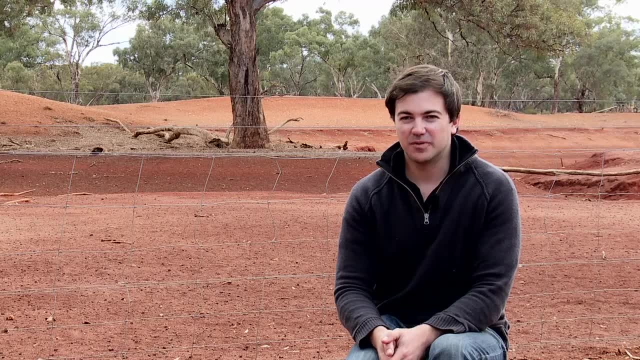 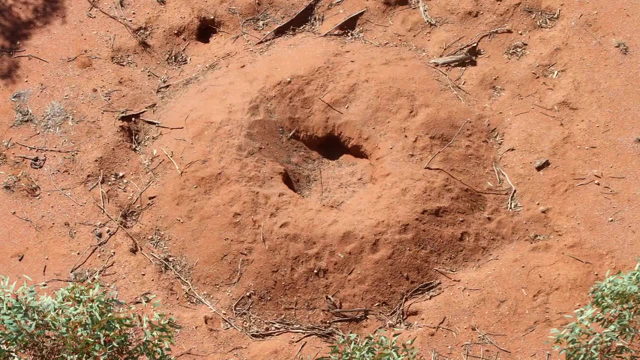 habitat degradation. so they'll turn over massive areas with their snouts searching for grubs and food, and they'll also trample the bush with their hard hooves, cause erosion, things like that, Predators as well of native species. so things like particularly the malefowl which we're 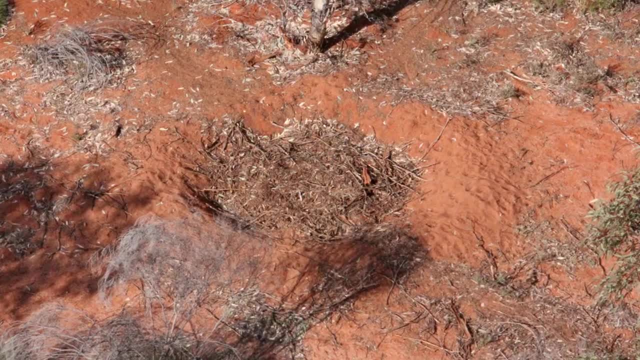 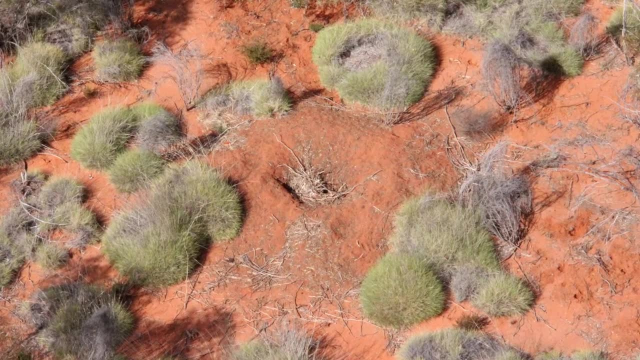 up here working on at the moment. they're a ground nesting bird, and feral pigs will wander along through the bush, find a nest, dig up the eggs and consume them. So what we've done here at the Invasive Animals CRC is we're going to be trialling the hog. 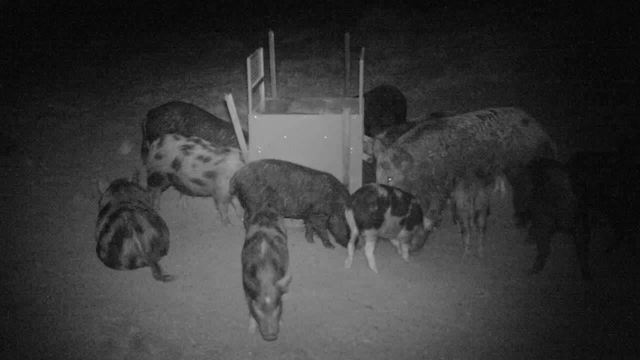 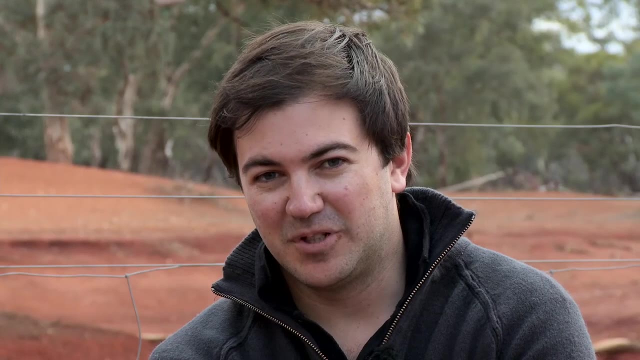 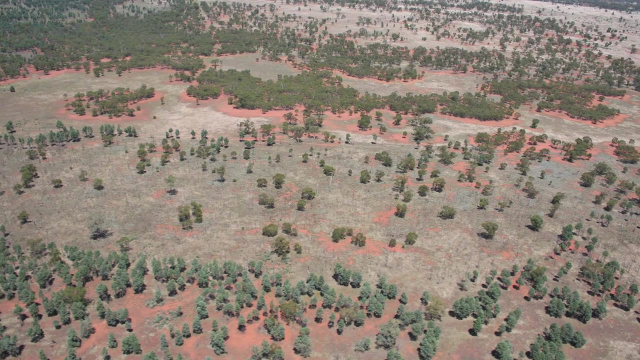 hopper up in this area to see if that works. designed specifically to deliver bait to feral pigs without impacting on non-target native species. The basic principles with pest management is to get as many people involved as possible. you want to broaden the target area cause that will help slow reinvasion if you only 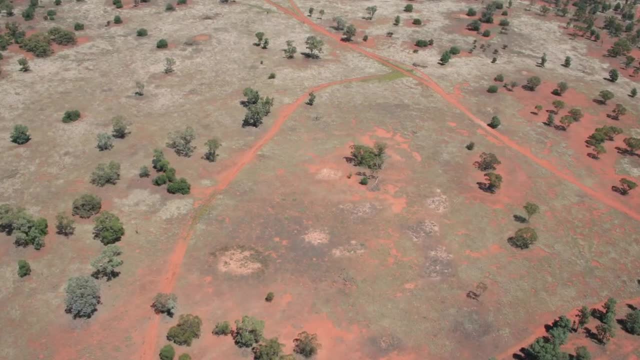 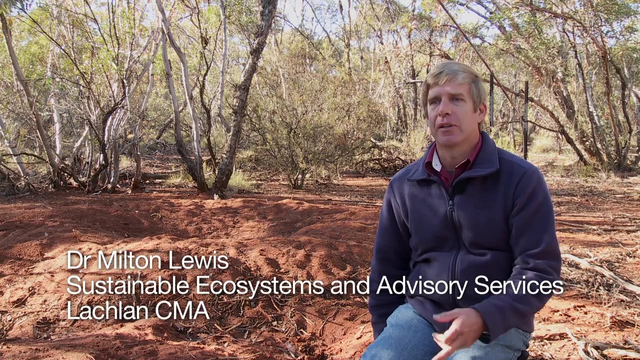 targeted one property in amongst a whole bunch of properties, you'll remove the pest from there, and then it won't be very long until they're all back in there again. We knew that helicopters were used fairly regularly in Yathong to check mounds, so we 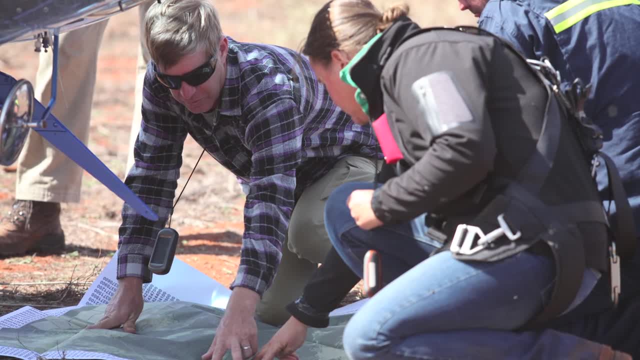 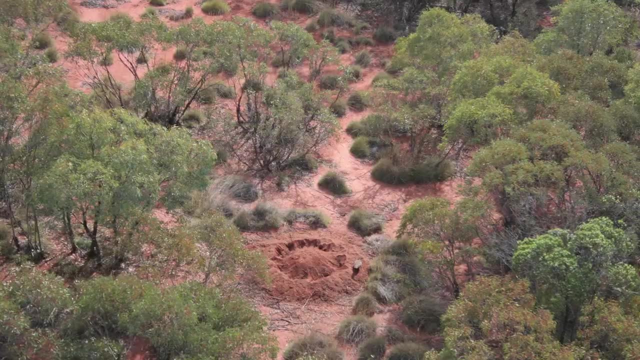 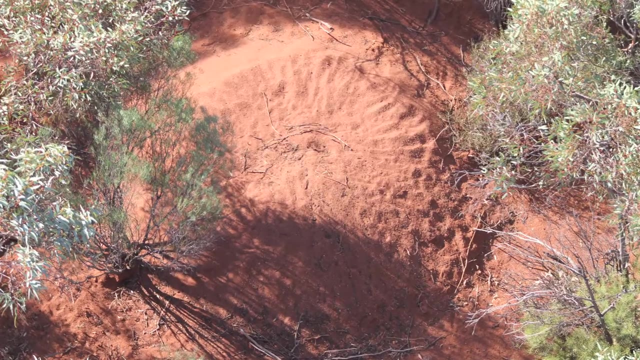 decided to try it for ourselves, and now we've covered over 100,000 hectares of mallee. We have about 56 active mounds currently And an awful lot more mounds that are not active, But some of those non-active mounds will become active in the future. 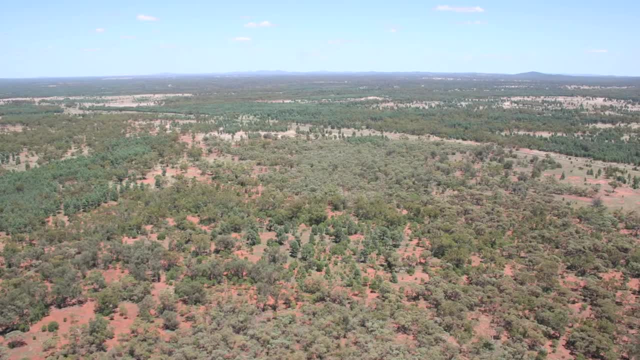 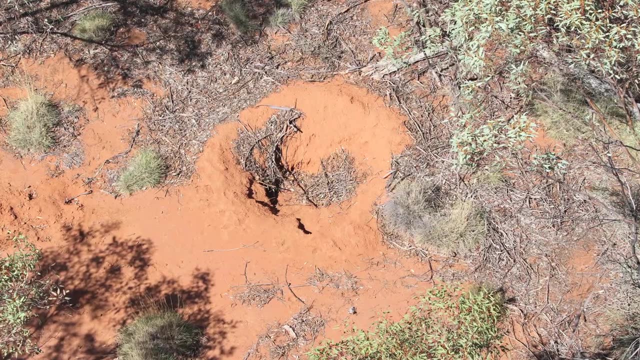 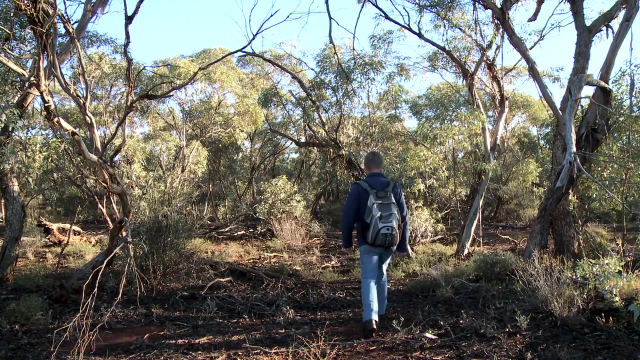 By flying the area we've saved an enormous amount of money and time. We can do areas in a week that would take us 12 months with 10 volunteers walking, And it's safer because this is difficult to work in The fencing in itself. 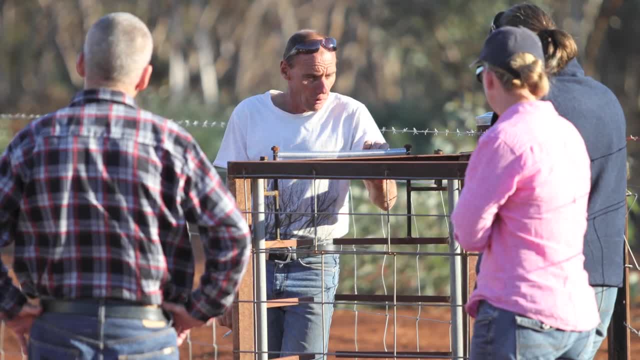 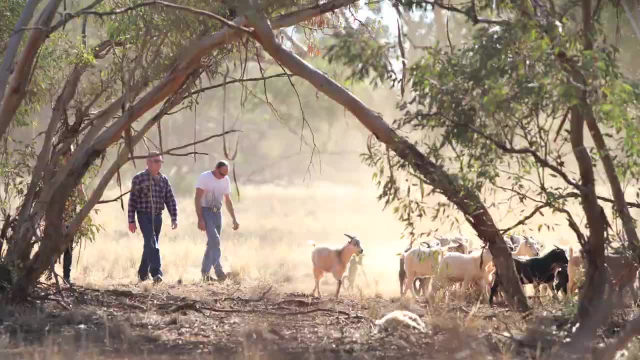 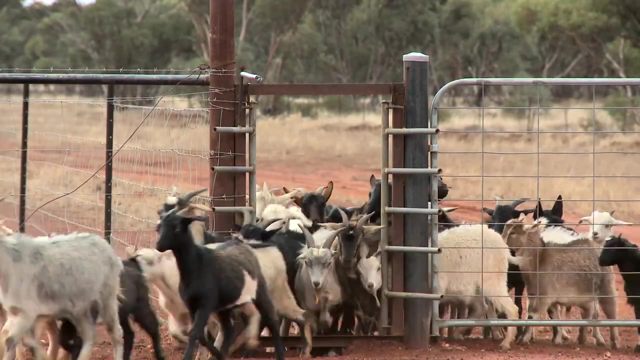 Has had the most dramatic impact on reducing the grazing pressure for the mallee fowl. So I think the most important thing we've done in the last few years is start a program of actively helping people manage the feral goat population here. The goat population has skyrocketed in recent years from hundreds to thousands. 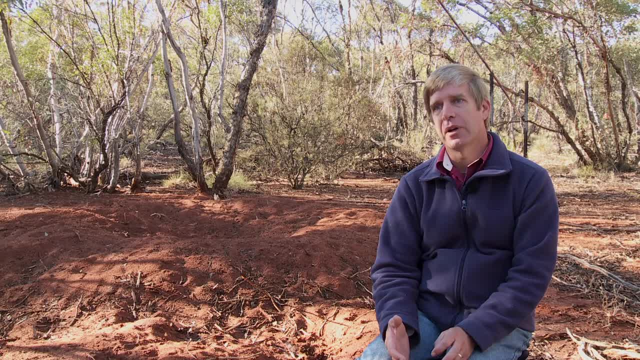 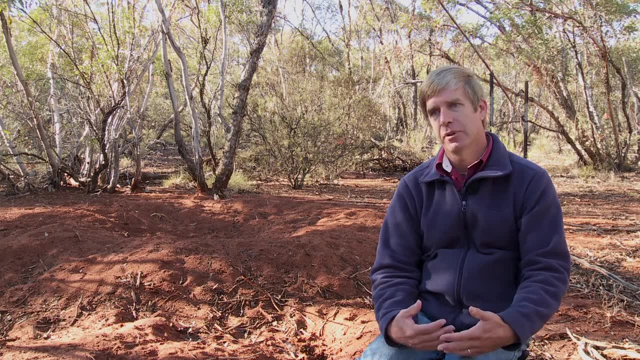 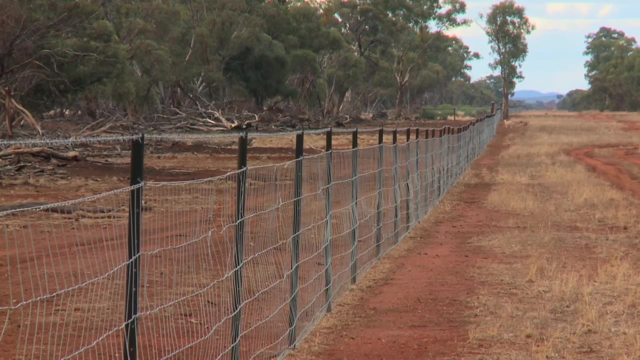 What we've done initially was we've put in 56 goat traps Strategically Across Our band through Mount Hope, To try and stop a southward progression of the goats. That was then followed on by what I think is a really innovative process of fencing. 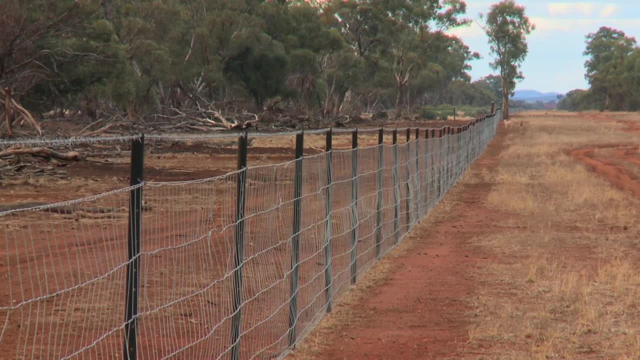 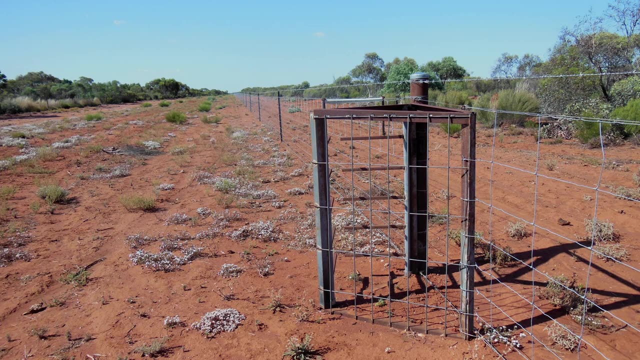 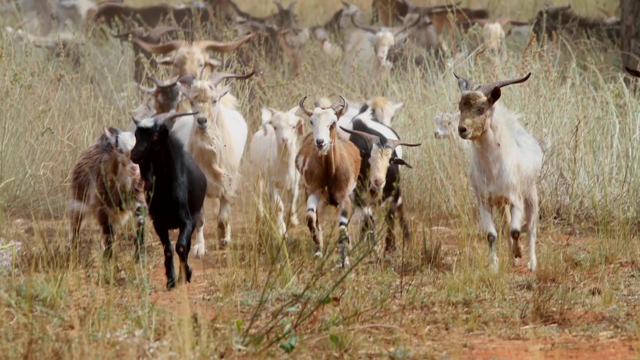 Where we've now started fencing areas that contain active nesting mallee fowl With a fence that contains one-way gates. So the mallee fowl are inside the fence. There are goats inside. The goats Leave to go to water Through the one-way gates. 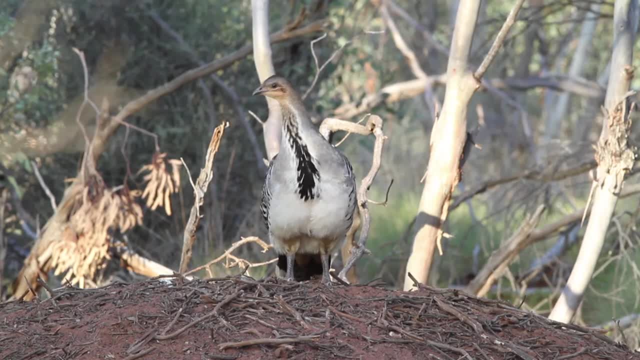 And then can't return to the mallee fowl. So eventually we empty the sites with the nesting mallee fowl of all the goats And therefore stop the competition between the two species, Because goats eat the same thing as the mallee fowl. 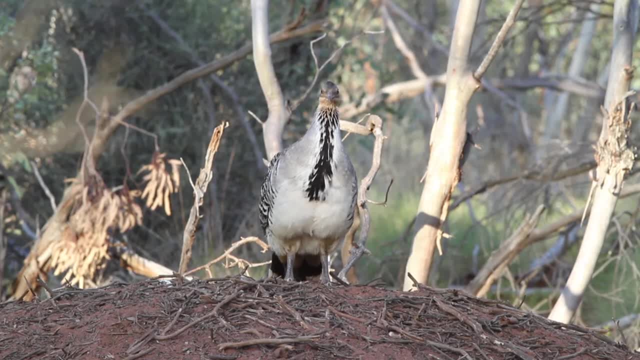 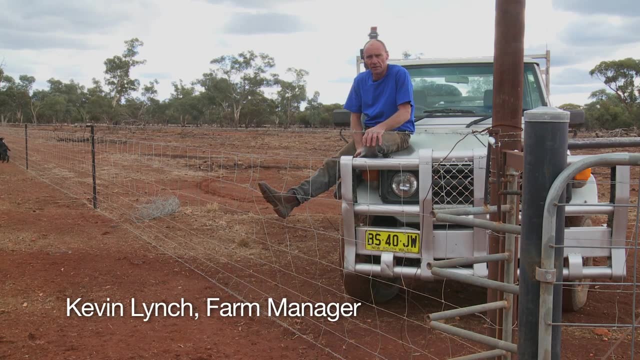 Be more of the landholders You know Need to understand what mallee fowl they've got there and understand what mallee fowl they've got, What goats they've got there, And get rid of the goats. The mallee fowl's going to do a lot better. And everyone does a lot better when you can get rid of the goats. So they're worth $1.85 a kilo at the moment, So it's not too bad of money. So they're worth chasing anyway. It's probably in the last five years, I suppose I've been running around chasing goats. 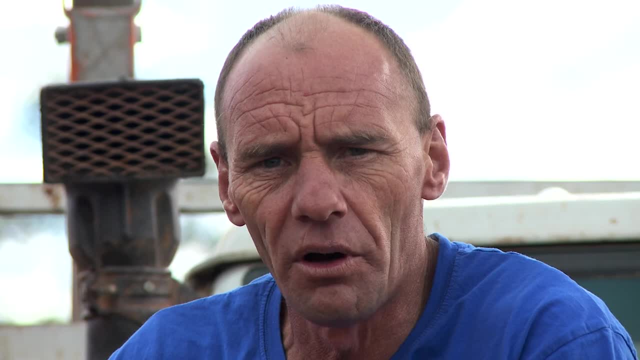 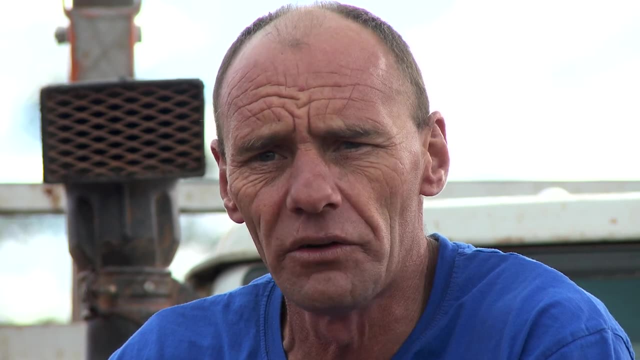 And yeah, it's helped my income a lot because I cut the broom bush here and now sort of. you know I've just backed off a little bit So I've just been doing goats and that's sort of the only income I've got at the moment. 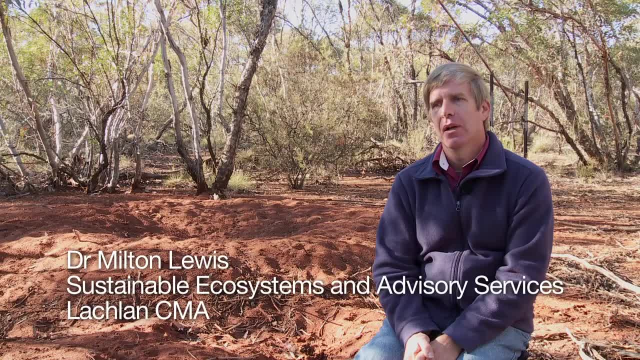 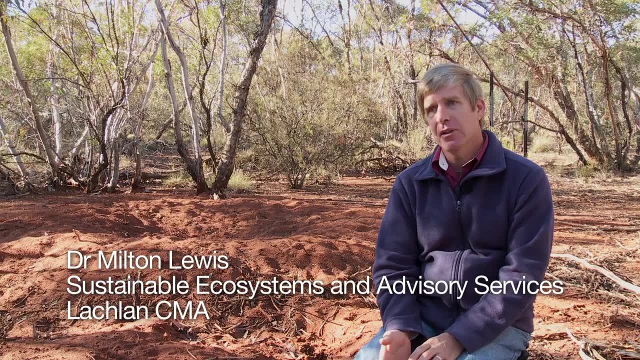 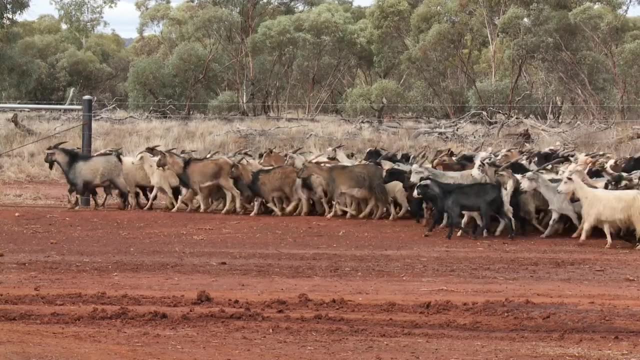 So it's yeah, it's helped me a lot. so The strange thing here is that a lot of people know that there are goats in the system, They recognise the goats are eating things, But some people haven't recognised that they were actually competing with their own sheep. 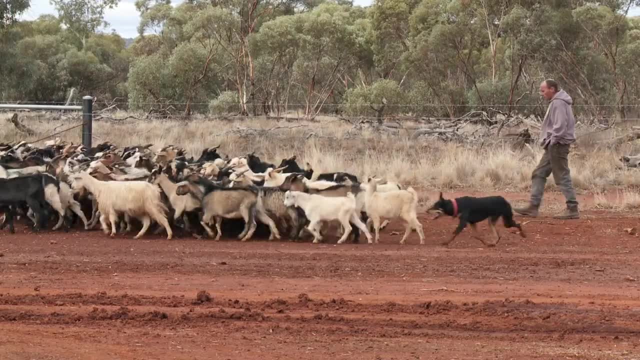 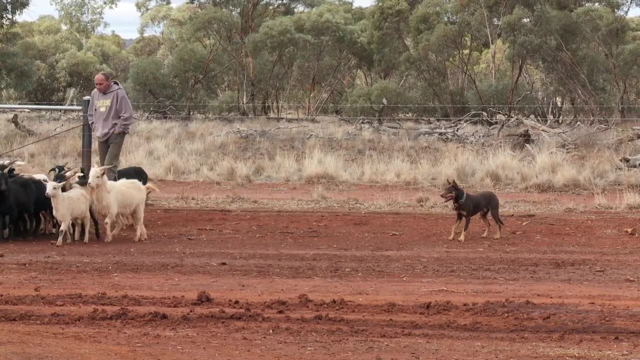 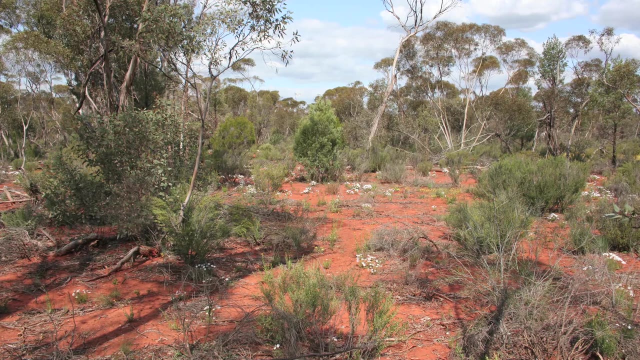 and cattle, But there are many more goats in here than there are domestic stock, Yeah, So in actual fact, their impact is much greater than any domestic stock have ever been. I have seen an enormous change in the structure of the vegetation since we've been reducing. 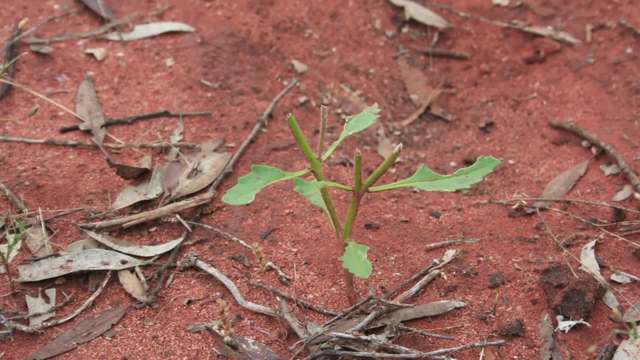 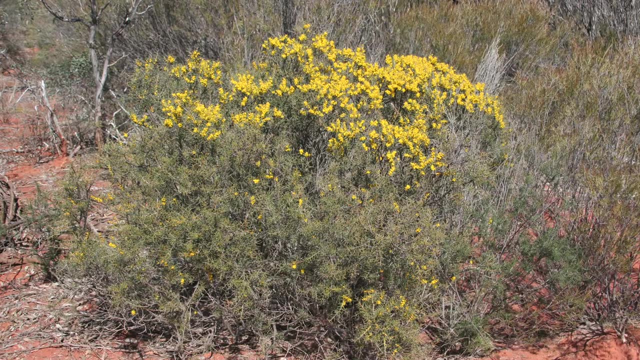 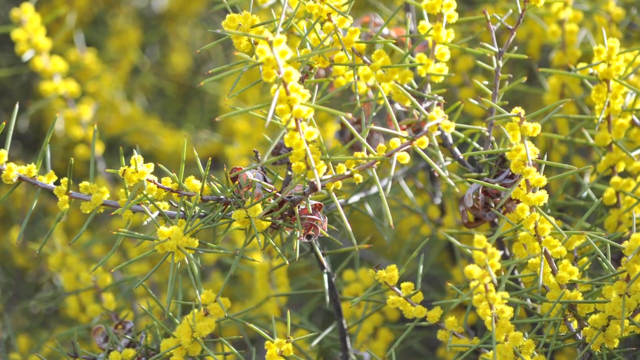 the impact of the goats. I used to walk through here and see shrubs eaten basically back to bare sticks. In the sites where I've been able to reduce the goat numbers, I've seen the regrowth on all of the shrubs to levels we didn't think were possible. 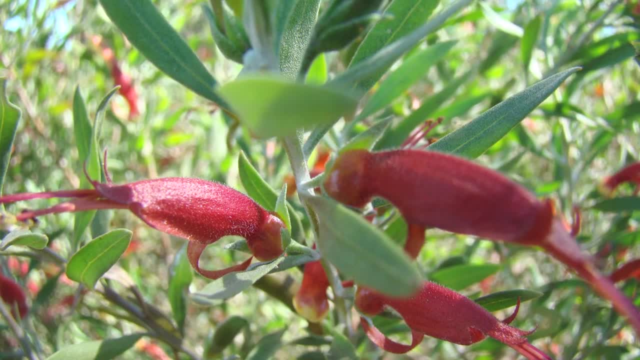 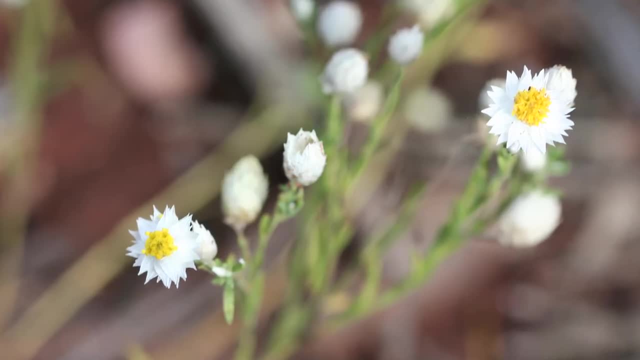 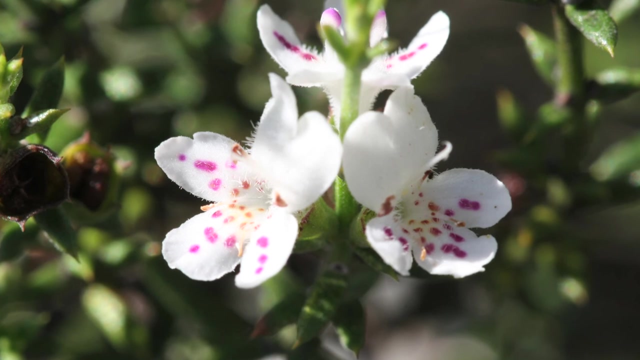 This isn't just about the mallee fowl itself. now This is about the vegetation right throughout Australia. The first thing is be aware of how much damage feral animals make. We often don't see them. They're cryptic, They sit in the background and we don't think much about them. They're just an opportunity for sport Mostly, But these animals are destroying the environment. Goats are eating it out, Foxes are eating our mammals and birds, Cats are just ravenous and taking lots of reptiles and birds out of the system. 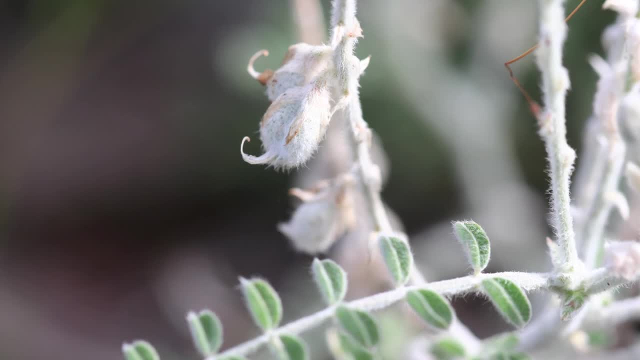 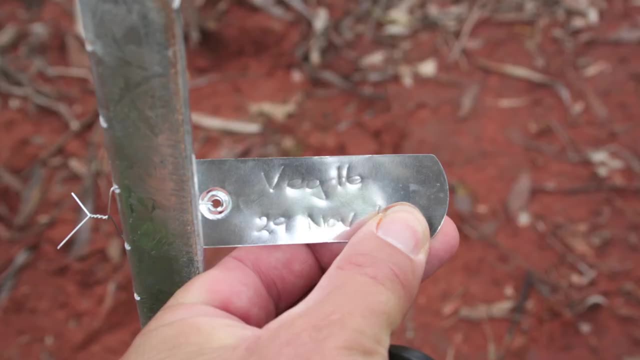 We need to be really aware of that and make sure we put in control measures for those animals And back the people that are trying to do the work. Too often we just don't get any help When we're trying to do the work. 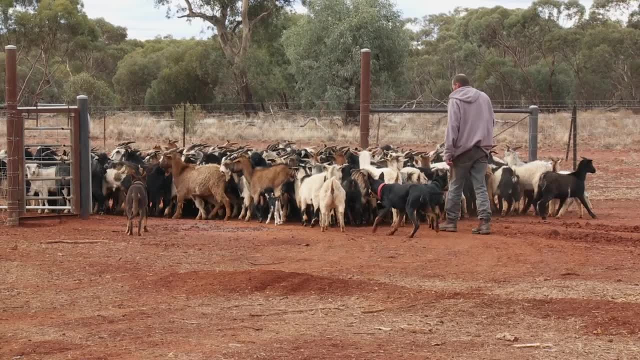 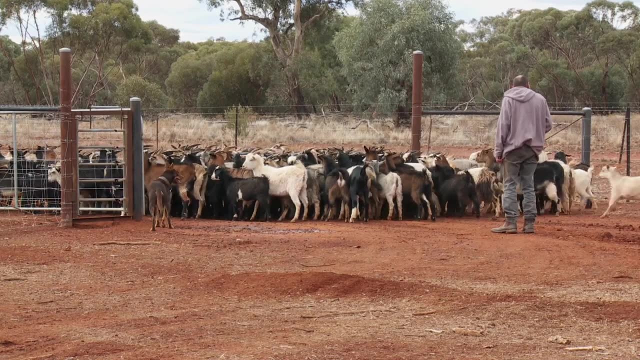 Yeah, We're trying to do what's best for the country And often we can make it financially worthwhile. The harvesting of goats has been amazing for people here. It got them through the drought. If it hadn't been for goats, many people would have had to walk off the land here. 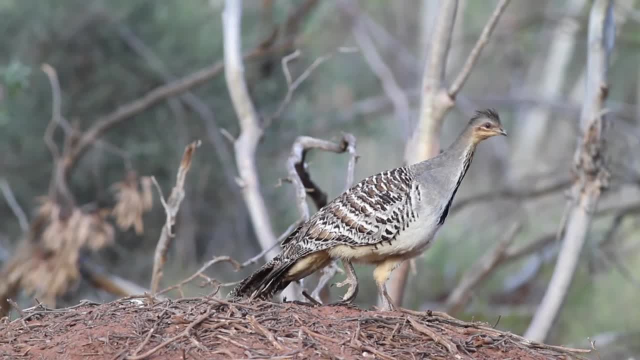 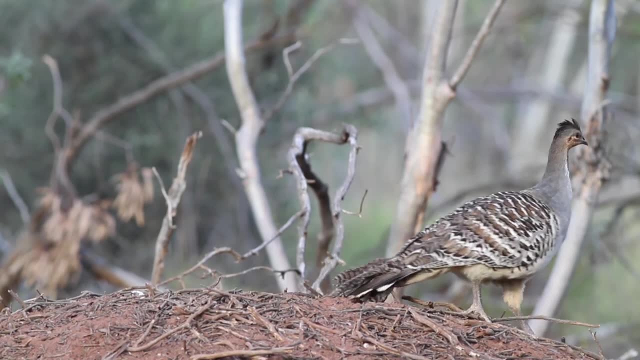 You know, early morning, late of an afternoon, you'll generally always see a mallee fowl, But sometimes they go quiet, like when they're probably nesting season and things like that. They're important to everyone, like I say. People just don't understand.